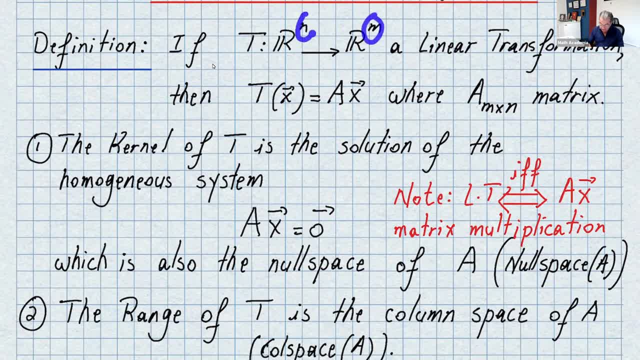 And please be careful, it's an m by n matrix And I put the note here for you. And in the last video we saw we have a linear transformation if, and only if, you can perform the action by a matrix multiplication. So there is always a matrix involved in a linear transformation. 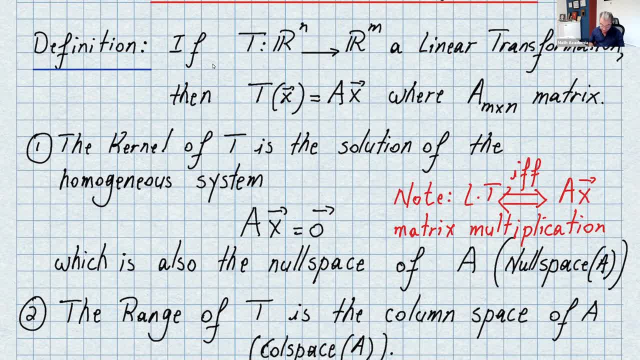 Now let's go over the kernel of T. So what's the kernel of T? The kernel of T is the solution of the homogeneous system. You take the same matrix, multiply it by x And you get the zero vector. we have seen homogeneous system in our last videos. 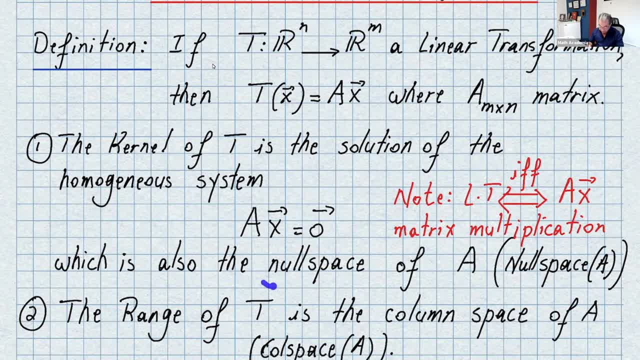 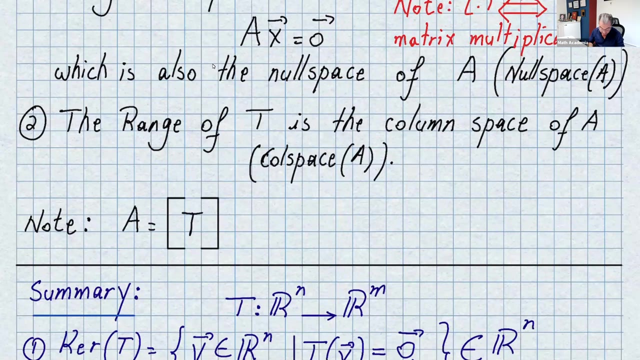 And, if you remember, this is also the null space of A, And I call that the null space of A here. So whenever you want to find the kernel of a linear transformation, you just find the null space of that given. Now, what is the range of the linear transformation? 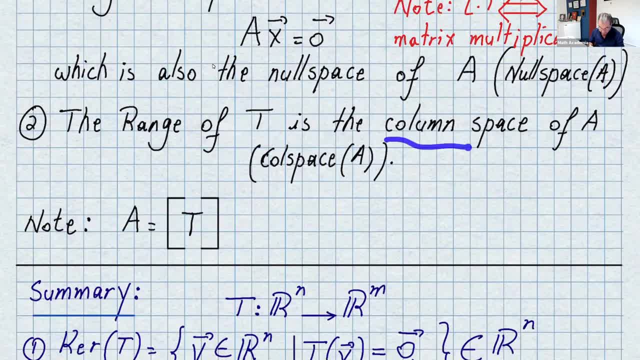 The range is just the column space of A And we can call that the call space of A. One thing to notice here. you're going to see sometimes A in the notations and sometimes T. These are the same matrix, So I did put a summary here. 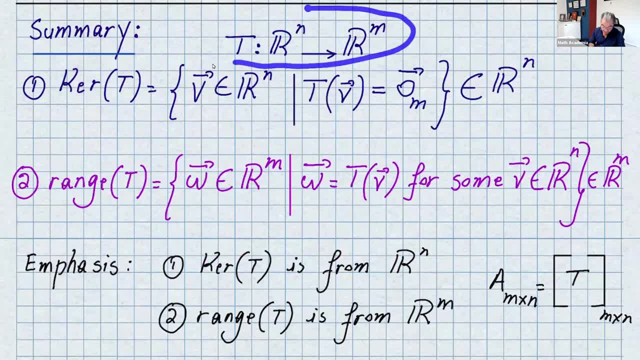 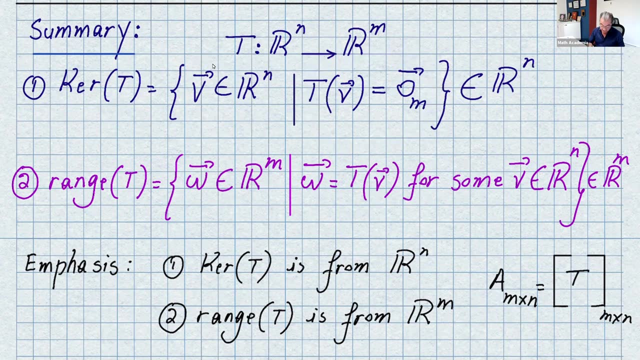 We have a linear transformation That's from Rn to Rm, The kernel of T. these are vectors in Rn And that's how you write it Basically. when you write the homogeneous system, that's T of equals to 0m. 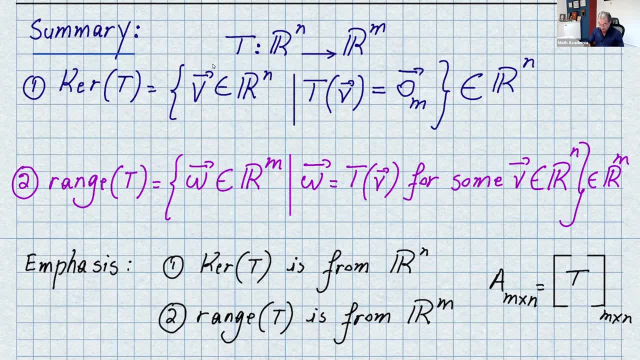 And please remember that's in Rn. in the example that is coming I'll show it to you. The range of T, these are some vectors in Rm where W equals to T of V, And again for some vectors in Rm, and that's in Rm. 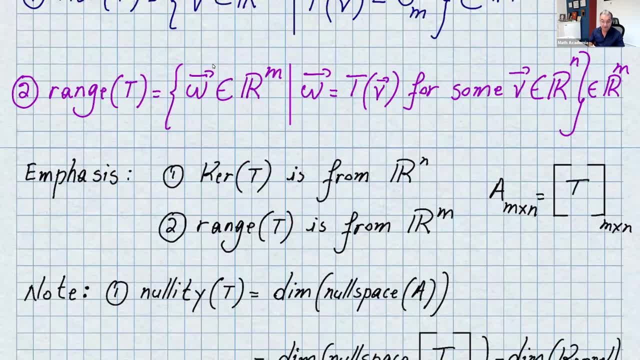 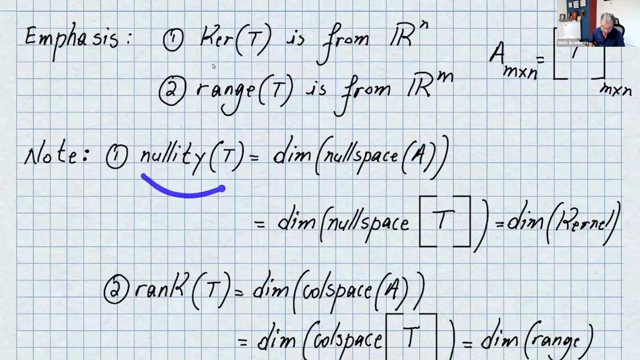 So the emphasis is very important here: Curve this from Rn and range of this from Rm. And don't forget Our matrix was an m by n matrix. I keep repeating that because it's important to know. Now we also have the nullity of the transformation. 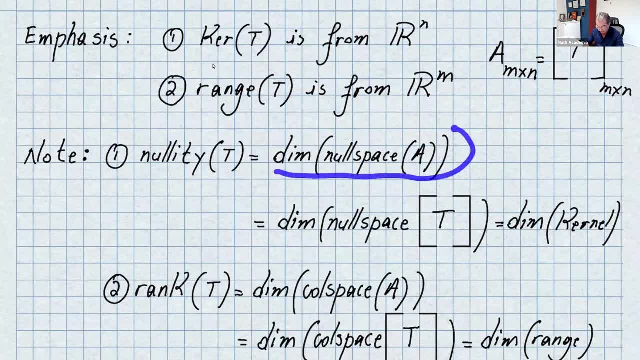 And that's just the dimension of the null space. As we noticed, the dimension of the null space are the vectors in the basis of the null space, the number of vectors And this is also again you can see A or T, the notation. 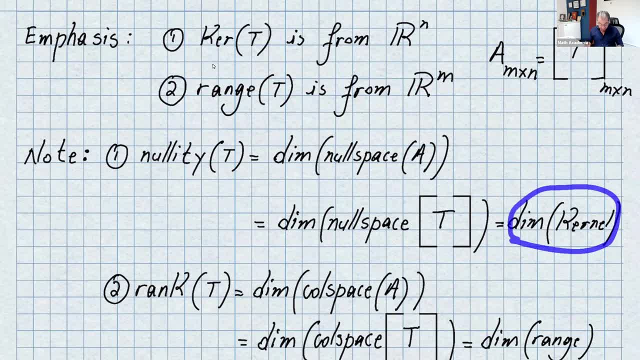 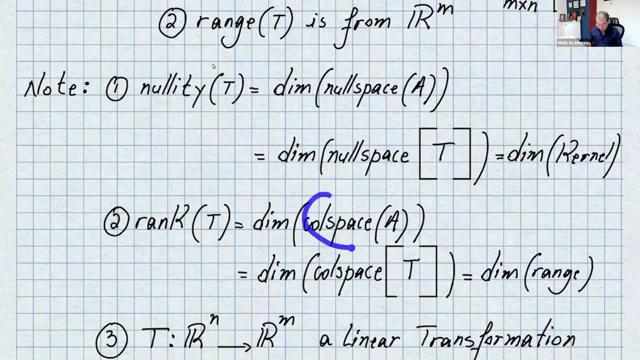 And that's the dimension of the kernel. Rank of T or rank of the transformation is the dimension of the call space, Again the number of the vectors in the basis of the call space of A. You can see also that notation. That's called the dimension of the range of the transformation. 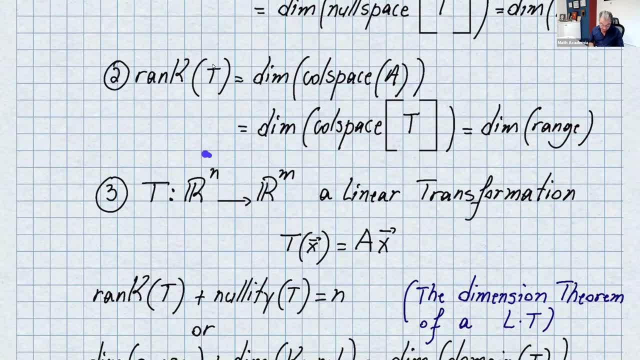 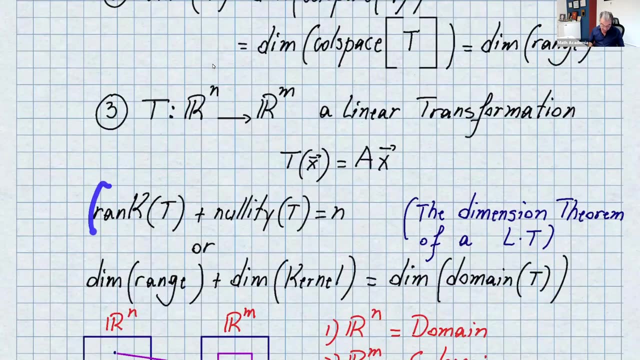 Now number three. if you have a transformation again from Rn to Rm is linear. of a linear transformation You can write: T of X equals to A times X. In this case, if you take the rank of the transformation plus the nullity of the transformation. 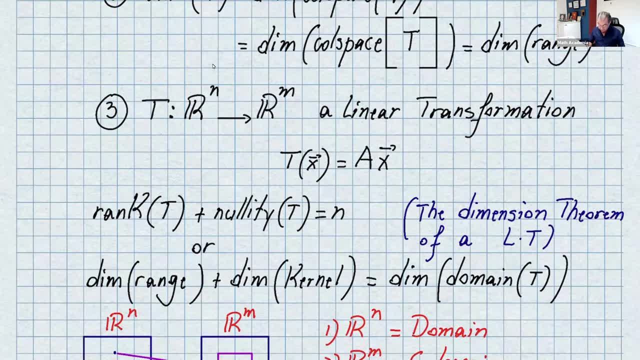 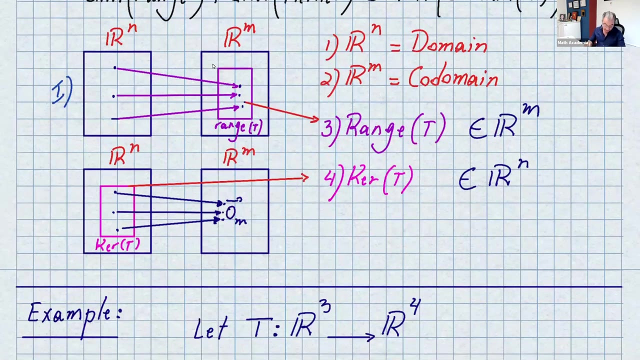 you should get N. That's the dimension theorem of a linear transformation, And this is the same thing as the dimension of the range plus the dimension of the kernel, And that's going to give you the dimension of the domain of T. Now let's see. if you want to kind of see the picture, 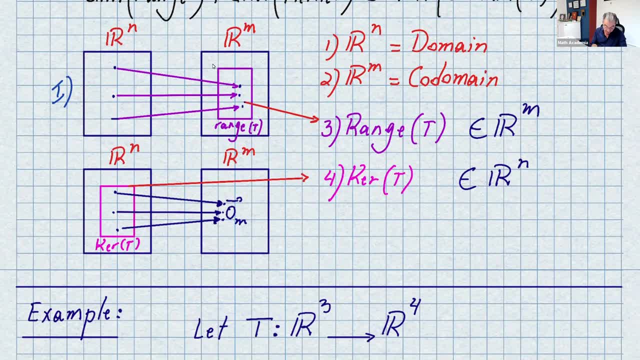 So again, here we have a transformation And we're going from Rn To Rm. The first thing to know, the domain of this transformation, that's Rn, The co-domain, that's what we call it, is Rm. 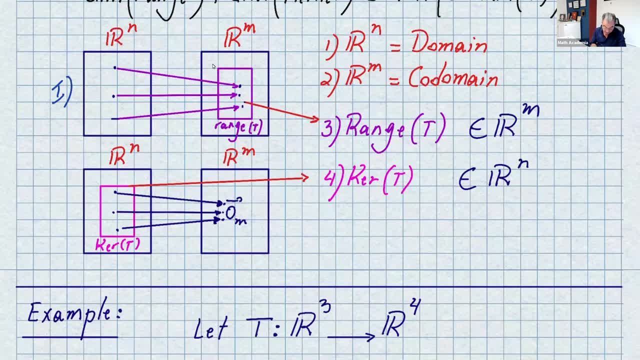 And sometimes they can be the same. I put the boxes the same size here, But in some examples you'll see how that works. Now, what's the range of T? These are some vectors in Rm So, and you see that those vectors are covering that. 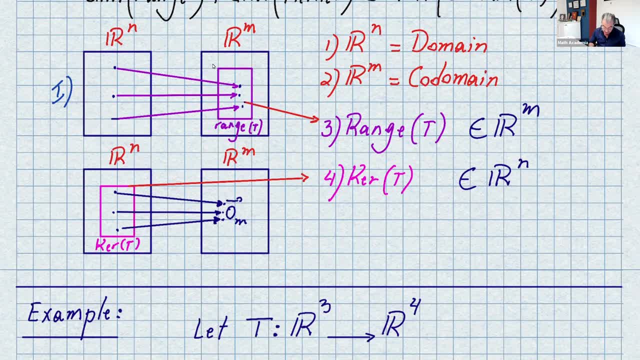 So this part is called the range of T. Sometimes the range of T can be the entire Rm And you'll see how that works and how we call that transformation. And I want you to notice also, range of T is in Rm, which is the co-domain. 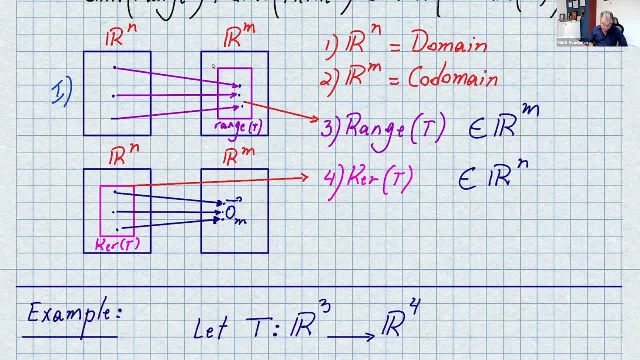 The co-domain of the transformation. Then we have- we can have here, Let me put number two here- Then we have the curve of T. Curve of T is right here And that's in Rn. So whatever vectors that make the transformation zero. 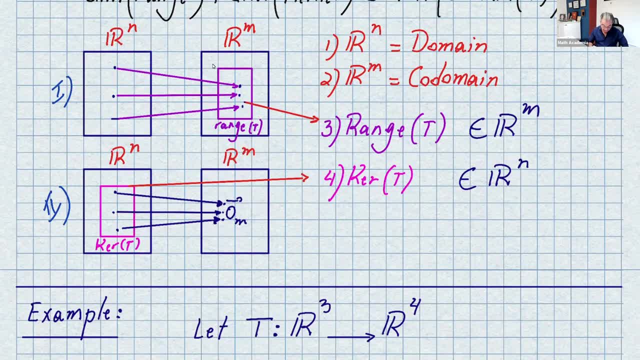 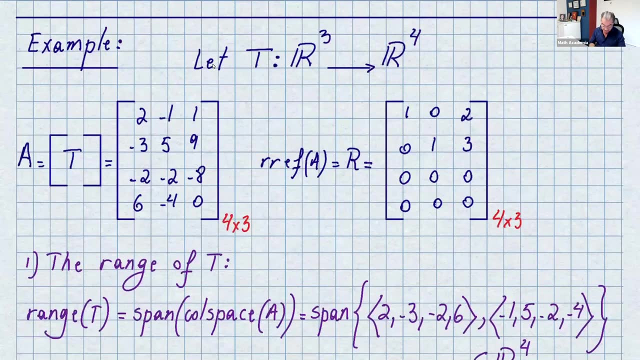 When you write the homogeneous system, So, and you get those vectors and that's called the curve of T. So let's do an example so you can see how this works. Let's say we have a transformation, We are going from R3 to R4. 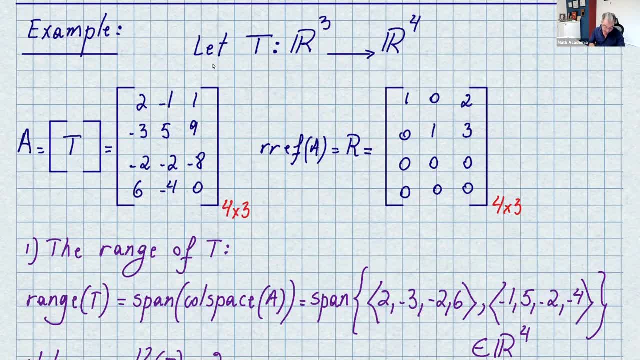 In this example, I, you are given the matrix A, Which is same as the matrix T. The first thing you want to do is find the RREF of that, Because all the information is you can get from the RREF of A or RREF of T. 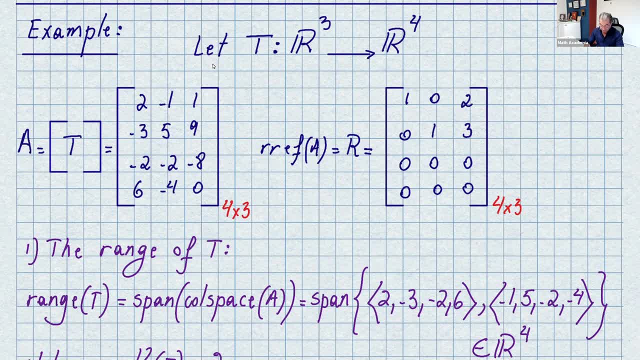 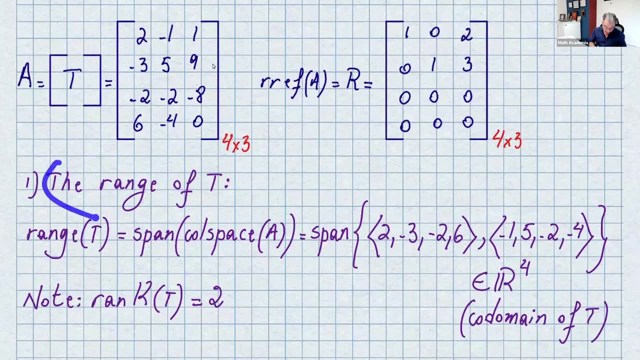 Just like last time when we were finding the null space, call space and the rule space of the matrix. It works exactly the same way. So now, if I want to find the range of T, We said the range of T is just the span of the call space or column space of A. 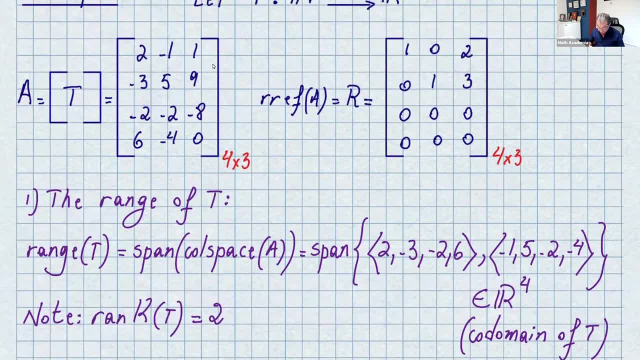 And the span of the call space of A, a basis in the call space of A here, Just like the last video I talked. So what you need to do is take the pivot columns And take the corresponding columns in the original matrix. 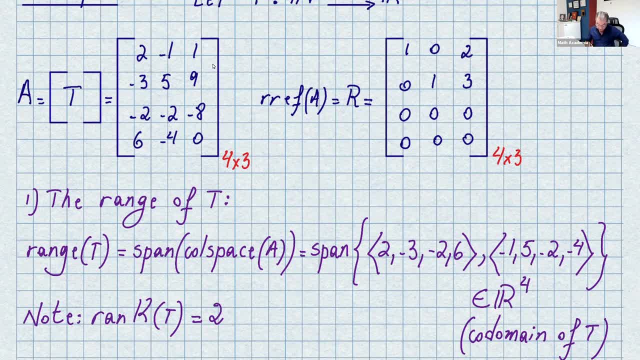 And these are going to be a basis for the call space. So I have two vectors here, So that's the first one And that's the second one. So basically, the range of the transformation is the span of these two vectors. 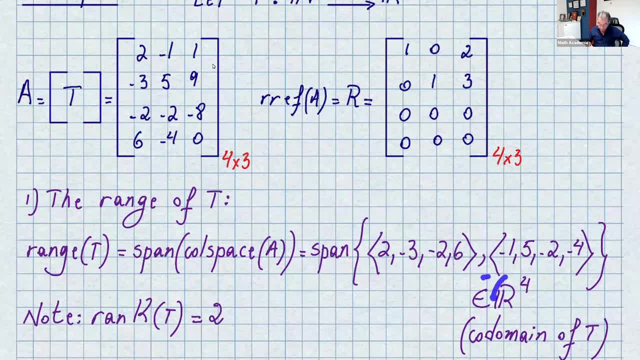 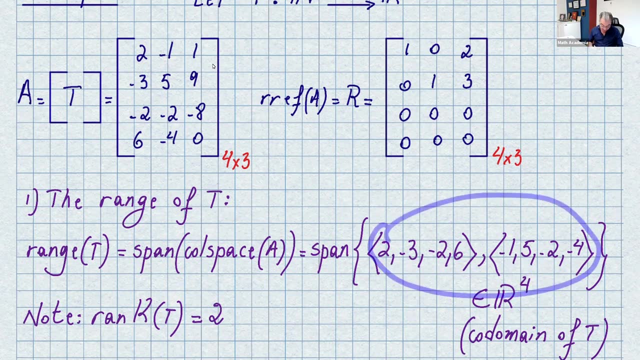 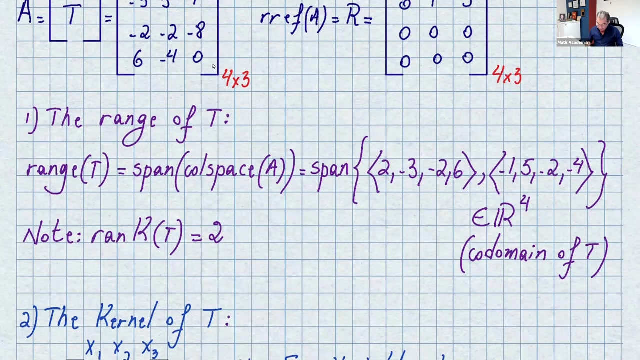 And, please notice, that's in R4.. So, as each vector has four components, Now if I say what is the rank of T? Rank of T is the dimension of these bases- We have two vectors And that's two. So, and again, this is in R4, which is co-domain of T. 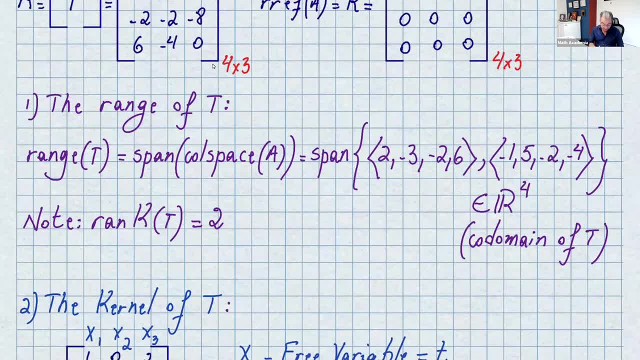 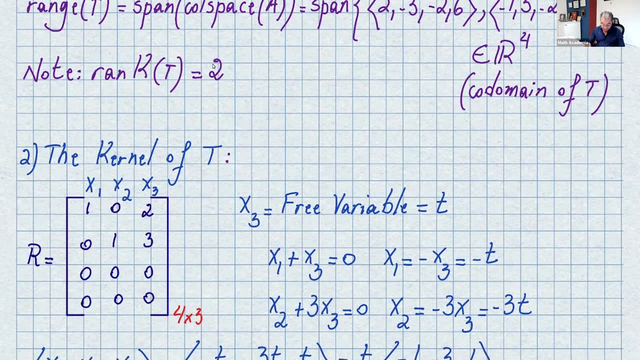 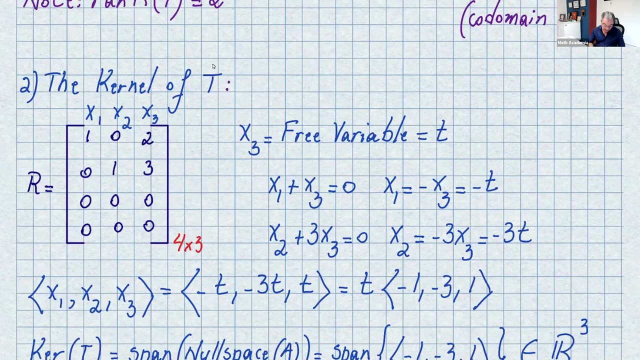 And it's right here, The kernel of T. All you do is to solve again, just like we did in the last videos and last lectures, The homogeneous system, So you can directly go to RREF. Here we see that we have two pivot columns. 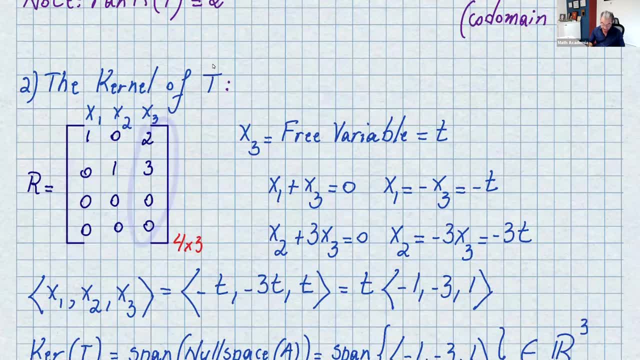 And this one is the non-pivot one. Therefore, that's X3 is the free variable. So you rewrite the system from here. You have X1 plus 2X3. And let me fix that. So that's going to be 2X3.. 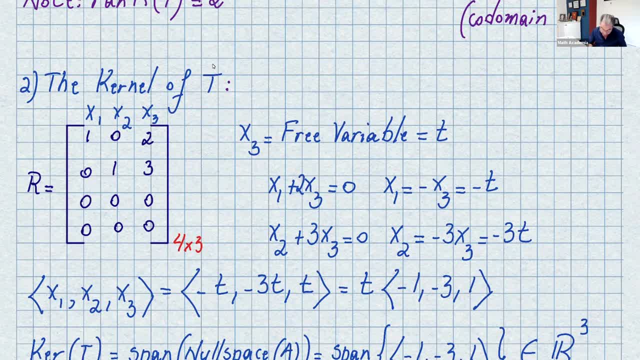 Which is, And then you can isolate. So that's X1 is going to be negative 2X3.. Which is the same thing as negative 2T, And from the second equation you have: X2 plus 3X3 equals to 0.. 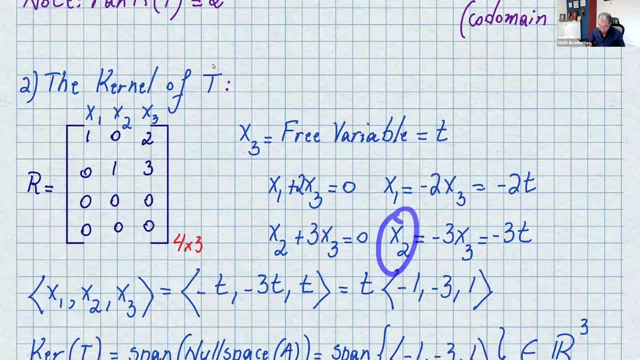 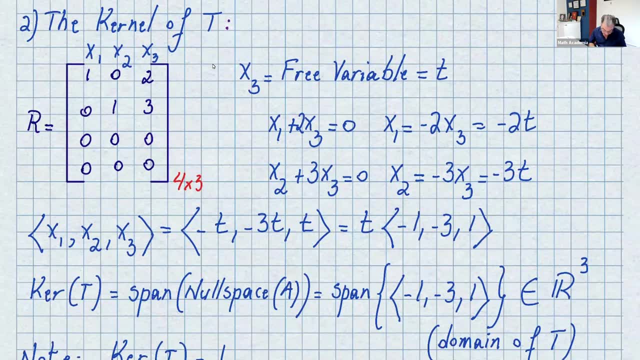 You isolate X2.. You get negative 3X3 or negative 3T. So if we come back and write this again, We know X1 is negative 2T And then we fix that, So that's going to be negative 2.. 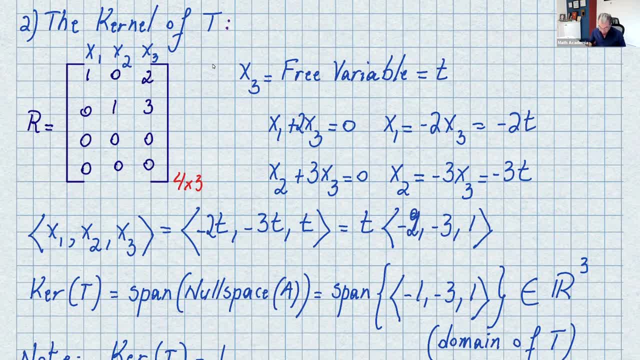 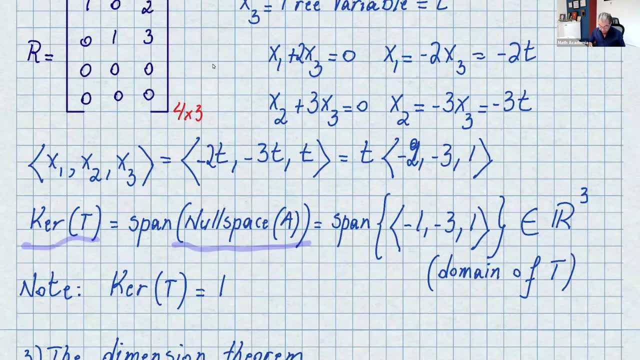 You can factor out T and you get negative 2,, negative 3, and 1.. So the curve of T is the span of the null space of A, as I said, And that's the span of a set, And this is in R3.. 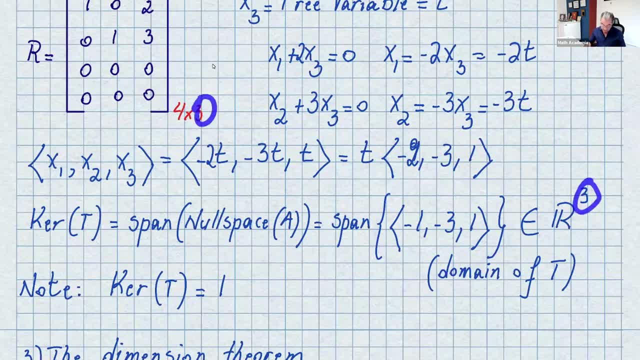 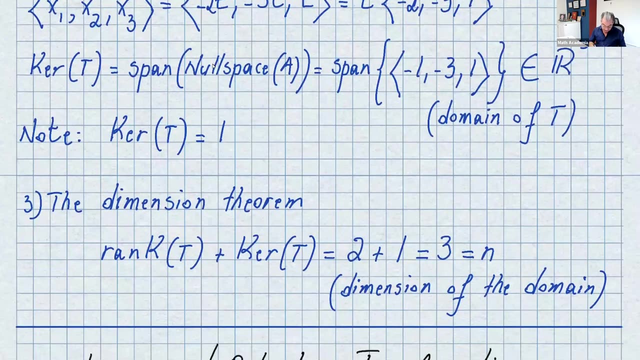 As we see it here, That's in the domain of T. Now the number of vectors in this space is 1.. So curve of T here is 1.. Now if we apply the dimension theorem here, We found the rank of T. 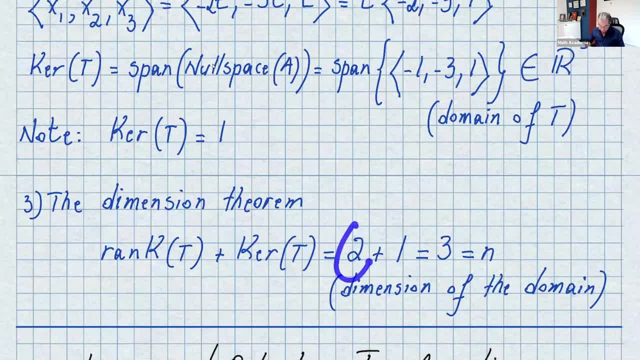 Which is the number of vectors in the call space, is 2.. And the curve of T is just the dimension of the null space, Or the nullity of T or A, And that's 1., And if you add them you get 3.. 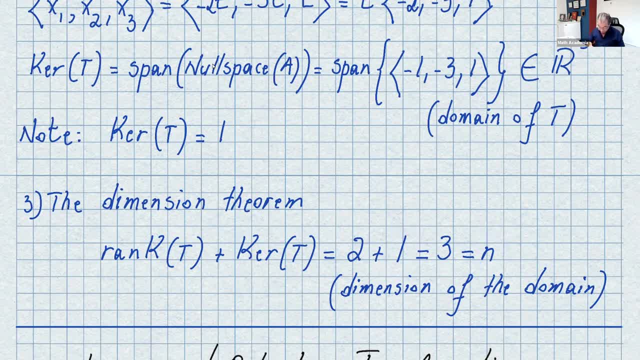 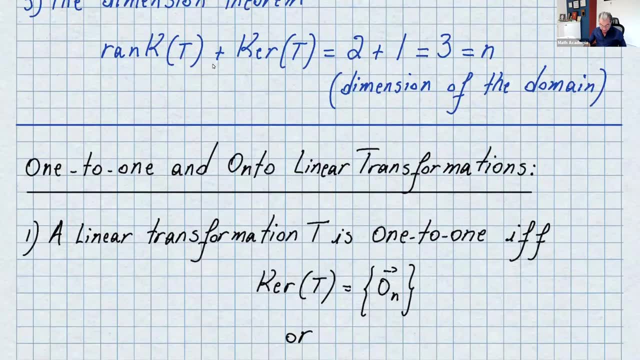 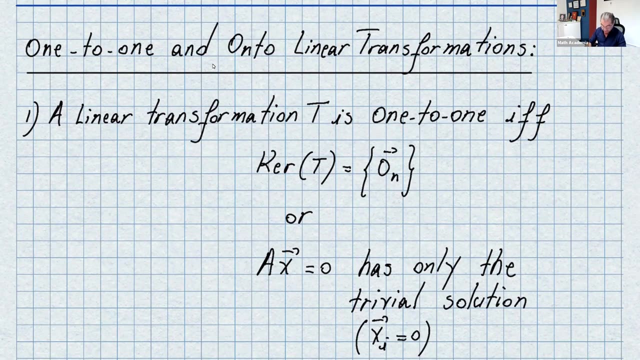 And that's the same thing as N, Which is the dimension of the domain. Now I want to just give you a little information About 1 to 1 and onto transformation, And in the next lecture, next video, I'm going to do a detailed work on that. 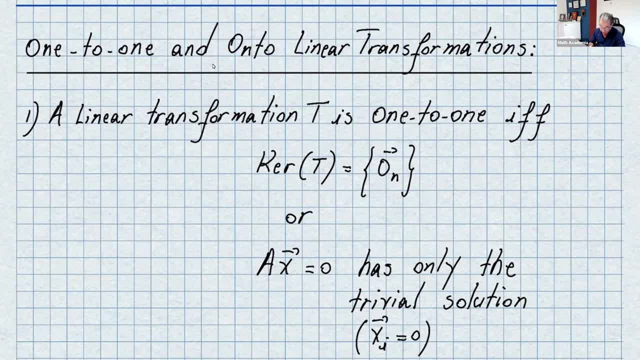 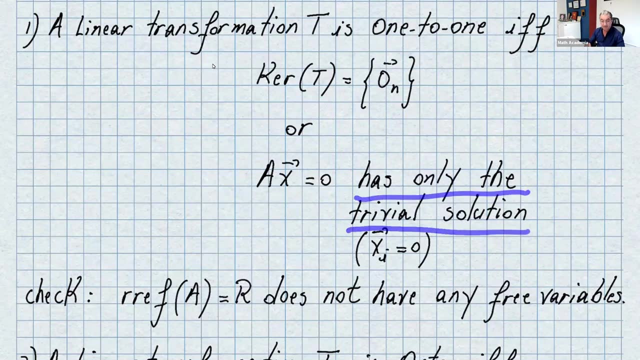 A linear transformation, T is 1 to 1.. If, and only if, curve of T is the 0 vector. So and what's the meaning of that? When you solve, AX equals to 0. Has only the trivial solution. So when that happens, 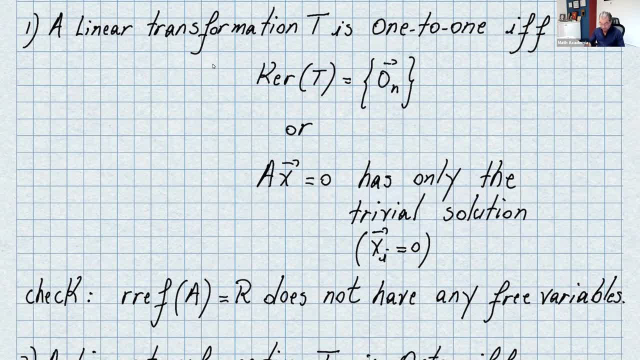 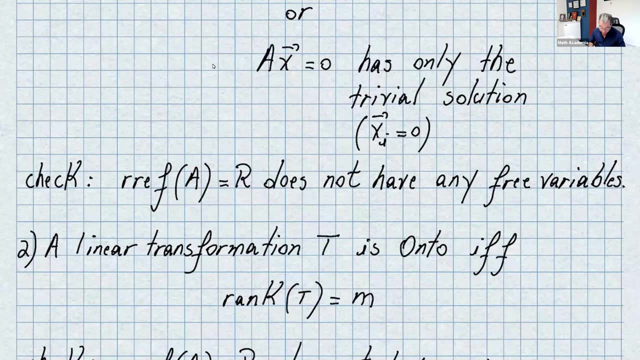 Then you can say it's a 1 to 1 transformation And what that is exactly. I'll go over that in the next video lecture. Now, if you want to find that fast, Check the RREF or R, And the RREF or R does not have any free variables. 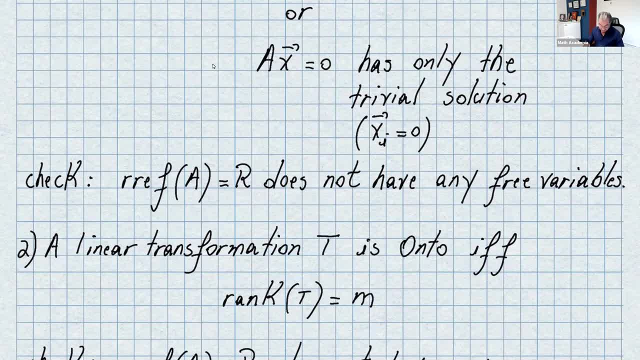 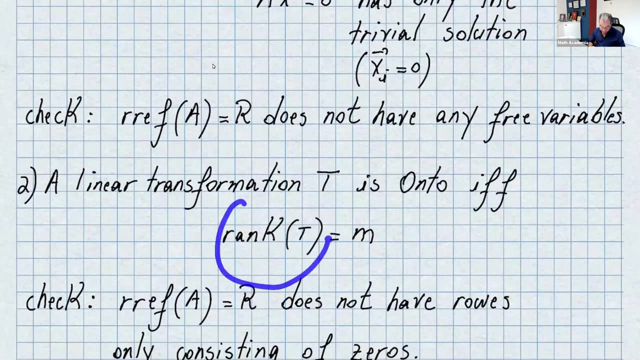 So once you do the RREF And you don't get any free variables, Then you can say that the transformation is 1 to 1.. Then the second one, A linear transformation. T is onto if, and only if, Rank of T equals to M.